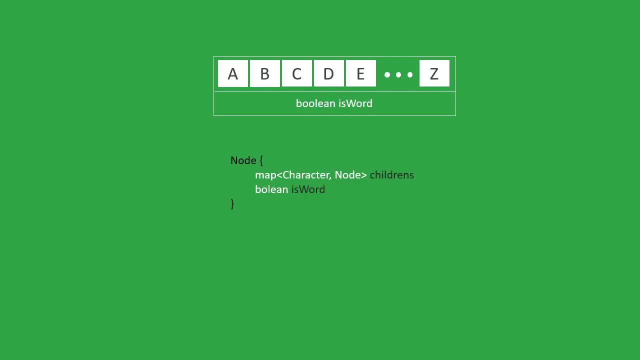 If you don't know what that is, imagine that you have table and each record contains character and corresponding node. Also, since the is word but also can be prefix to their, we have to be able to decide whether this word is in our tree or whether it is just a prefix. 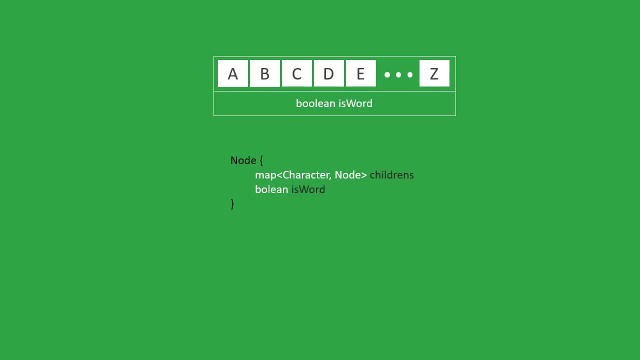 That is why we have boolean variable, which indicates that. Let me show you how you can add words. I got here my root name And words I want to add, So let's add car. As I said before, every node represent one character of some prefix. 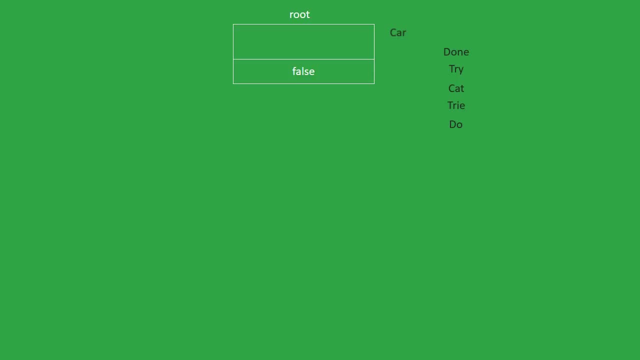 So we split this word in two characters And add to our tree prefix for every word starting with C Inside this node we want to add node that represents all words starting with CA. So we add A into its map and create a new node. 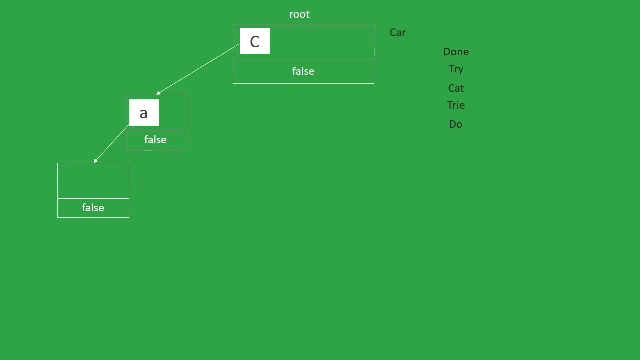 So this new node represents all words starting with CA. As you probably figured out, we add to its map R character And create a new node. This node represents all words starting with car. Since we want to add this word, we set its indicator to true. 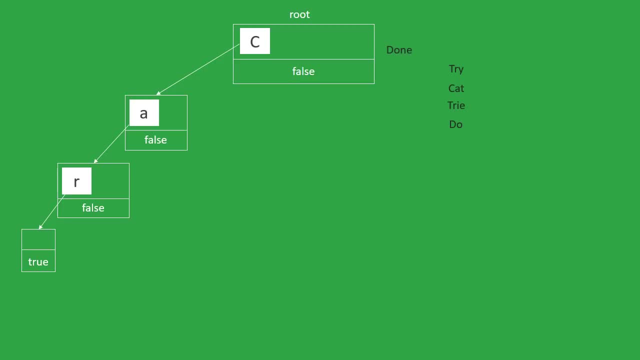 Let's try to add done So once again. we start at root and look at its table And see that we don't have any node representing the prefix. So we create one And add new record to root's map. In this new node we look for O. 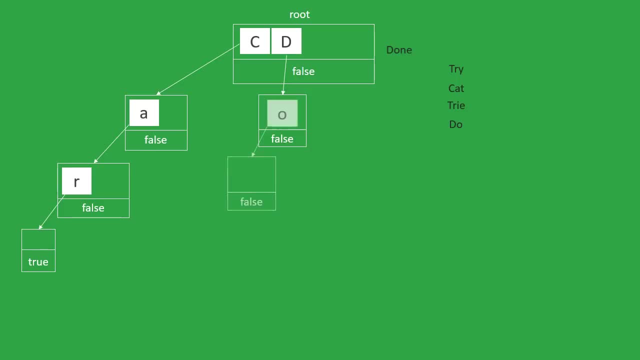 Since there is no O in our table, we add it and create new node which represents do prefix. In this node, we continue with N, where the same thing happened as we create new node for done prefix. In this node, we add E. 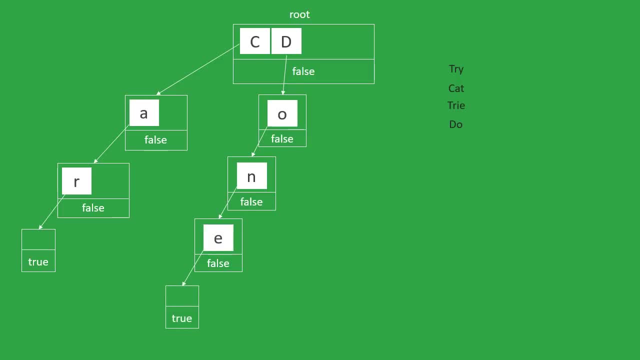 And once again create new node. And since we have no other characters in done, we set this node's word indicator to true And we are done. Let's try to add. try Once again. we look at root and try to find T in its map. 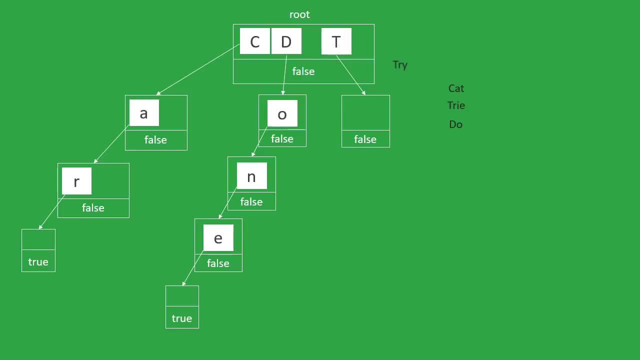 But T isn't there, So we create new record for T and add to it corresponding node. We move to this node and continue with next character, in this case R. Since this node map is empty, we add there R And create new node representing TR. 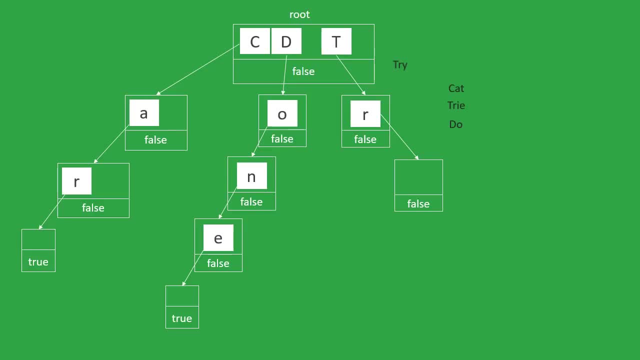 And we add to this node Y record, And once again we create corresponding new node. This node represents prefix try, And since this is the word we want to add, we set its word indicator to true. Now let's add cat to our tree. 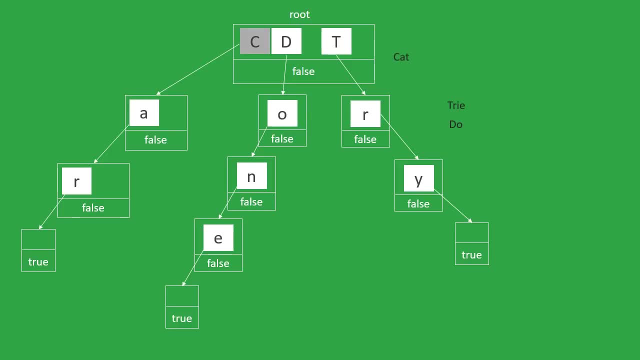 So we look at root. But we find out that C is already in our root's table, So we move to node representing C prefix. And in this node's table we look for A. A is already there, so we move to corresponding node. 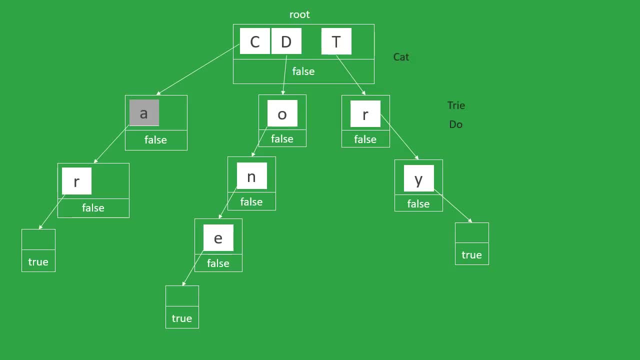 In this case, we look for T And we find out that T is not in our node. So we add T and create new node. And because we have no other characters in cat, we set the word indicator to true. Let's add try. 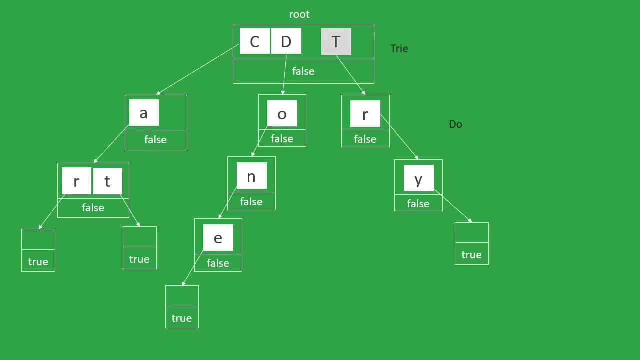 We look at root's table and find out record T is already there. We continue with corresponding node. In this node we find R and move to node representing TR prefix. Now we look at I in this node. Since it's not there, we create new record for I and new node for try prefix. 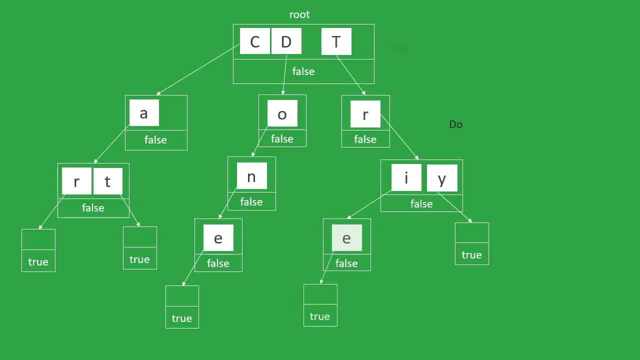 Since we still have one character left, we create new record for E and new corresponding node. In this node we set the is word indicator to true. Let's add our last word. do We look at root and see that D is already in the table? 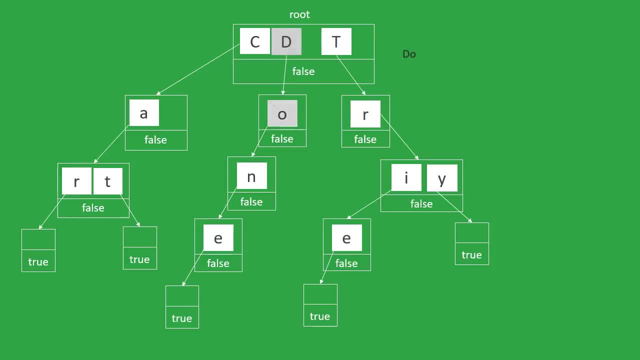 So we follow its pointer. Now we try to find O in this node. O is in this node, so once again we follow its pointer. Since we have no other characters to follow, we set the is word indicator of this node to true. 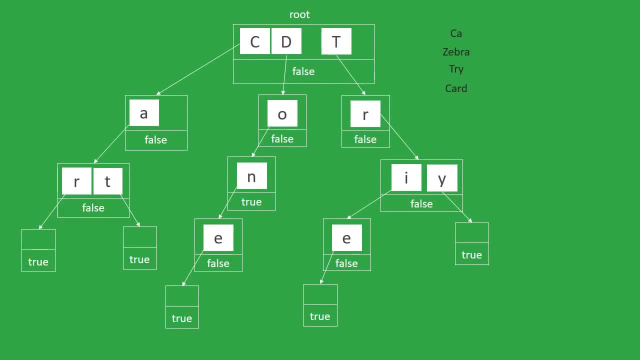 Let's try to find some words. First word is CA. Remember, each node represents prefix, So we start at root and look for prefix C. We follow C's pointer and in this node's table we are trying to find A, Because in order to find CA, we need to find CA prefix. 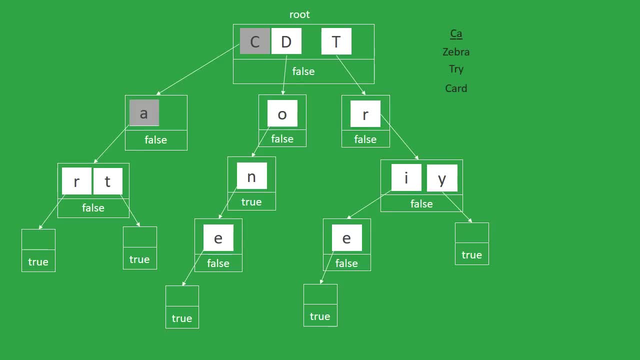 A is in table. so we follow its pointer and get the node which represents CA prefix. So we look at its word indicator and since it is false, this word is not in our table, Even though we found corresponding prefix. Let's try to find zebra. 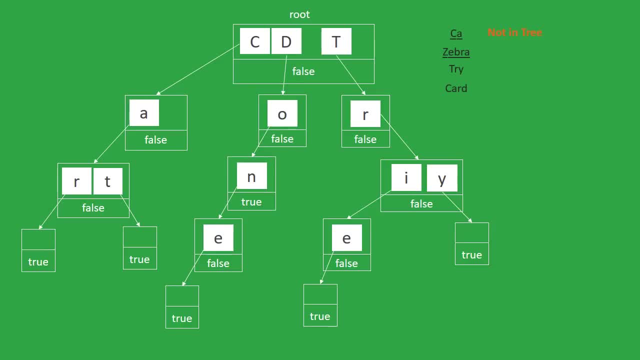 So we look at root's table and look for Z. Since Z is not in there, there is no way that zebra is in this tree. Actually, because Z is not in root, we can say that any word starting with Z is not in this tree. 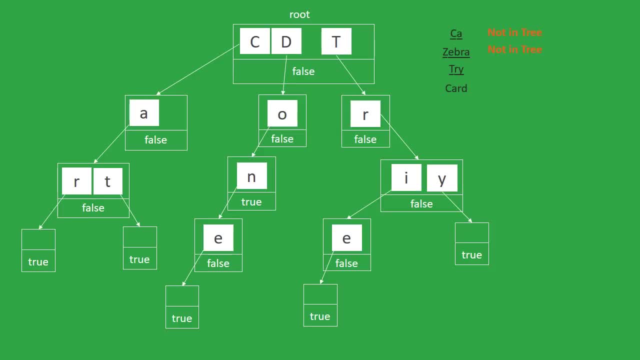 Let's find try. In this root's table we found T record, so we follow its pointer In this node. we continue with R. since R is in this node's table, we follow its pointer and get to node which represents TR prefix. 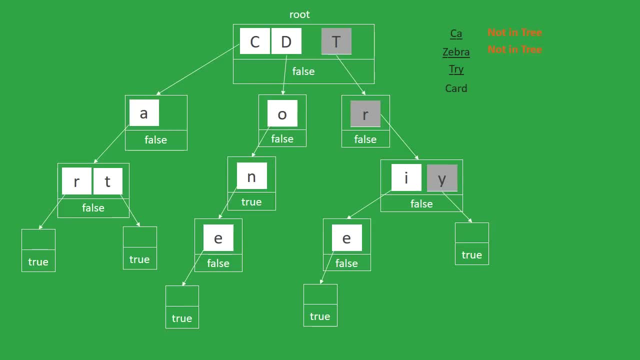 In this node, we look for last character I. I is in this table, so we follow its pointer, and since we have no other characters left in our word, we look at this node's its word indicator, Since it is true, we can say that try is in this tree. 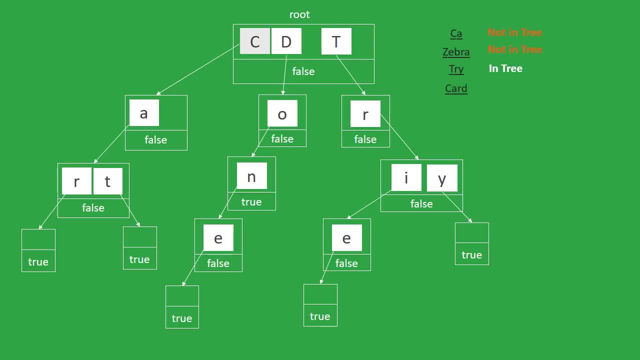 Let's try to find card. We start at root and follow C, Then we follow A. We still have two characters to go, so we continue with R. We get to node, which represents card prefix, and look for D in its table. Since it is not there, card is not in this tree. 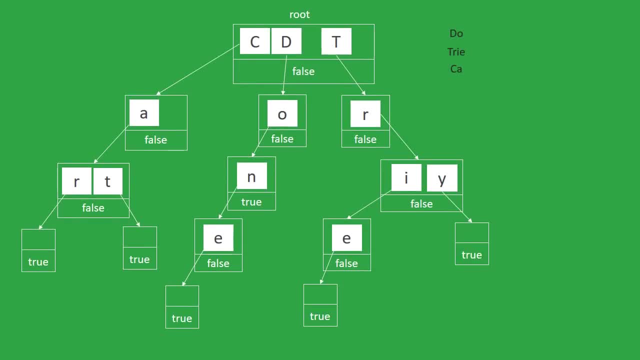 Let's try to delete some words. In order to delete a word, we need to find it. If this node have child nodes, we cannot delete it, So we just set ID. If this node have no childs, we can delete it. 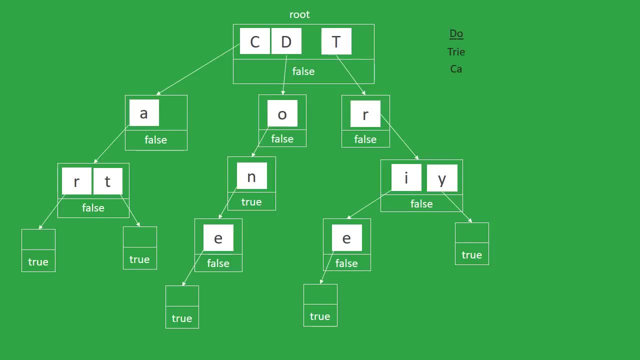 And then check if we can also delete the nodes above. So let's delete DO. We look up DO and see that the nodes representing DO prefix have childs. So we just set the its word indicator to false. Now let's delete TRY. We look up, TRY. 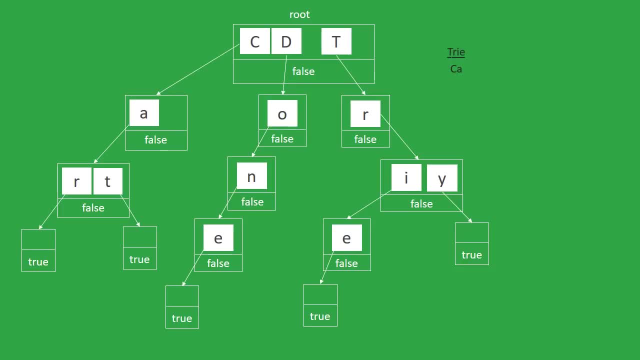 and see that the nodes representing DO prefix have childs. We look up, TRY and see that this is a leaf, In other words it has no child. So we delete it And also delete the record that points to this node in node above.